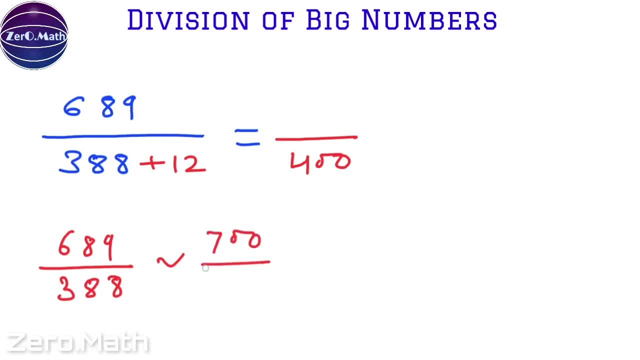 To find out what we'll do, we will find out the approximate unit value of 689 by 388.. 689 is approximately equal to 700.. And 388 is approximately equal to 400.. If you divide 700 by 400, we are going to get approximately 2.. 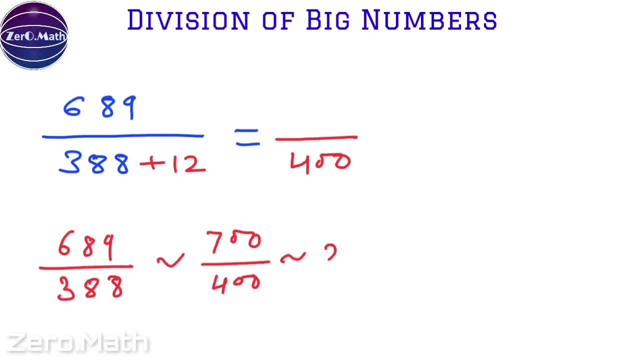 Because 4 times 2 equals 1.. So, compared to 7 is approximately 0.. So 388 is approximately equal to 300.. is 8, 400 times 2 is 800, so it will be approximately 2.. Since we are adding 12 to the denominator. 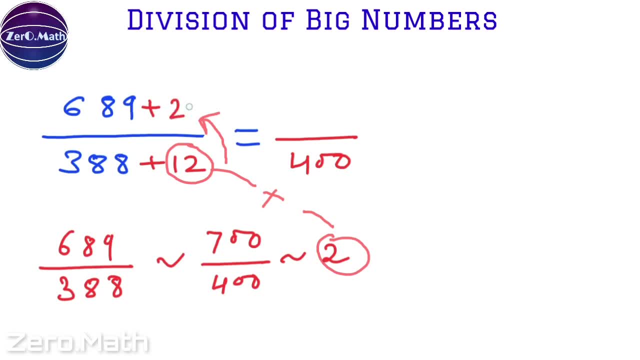 let us add 12 times this- 2 is equal to 24- to the numerator. So 689 plus 24 would be 713.. Now let us divide 713 by 400 to get our answer. So, since there are 2 zeros, I. 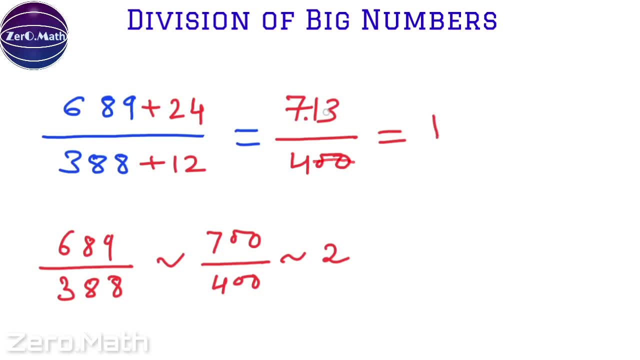 will give this decimal point over here, and 4 times 1 is 4,, carrier would be 3,, 3 and this one will be 31.. So 4 times 7 is 28, and carrier would be again 3, it will be 33. 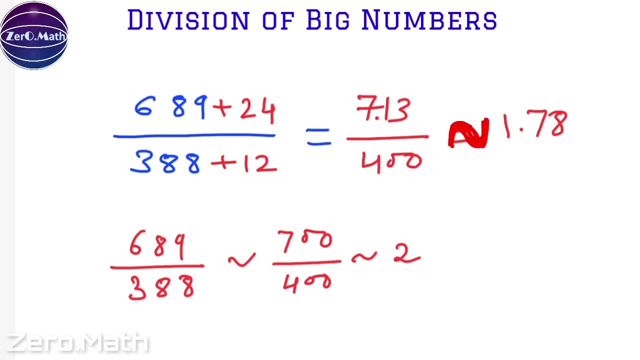 now. So 4 times 8 is 32,, carrier would be 1.. So I will give 0 on that, 1.. So 4 times 2 is 8, carrier will be 2, 20, and 4 times 5 is 20.. 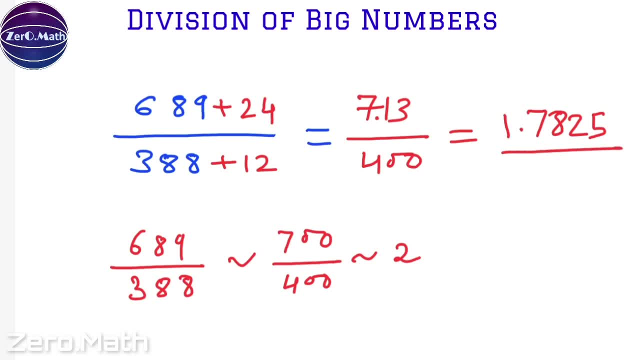 So 1.7.. 825 is precisely our answer. Now, if you try to find out the answer with the help of calculator, you will get 1.7757, and you can see there is hardly any difference. So 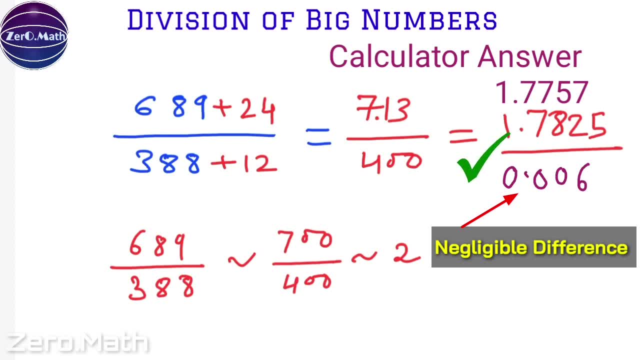 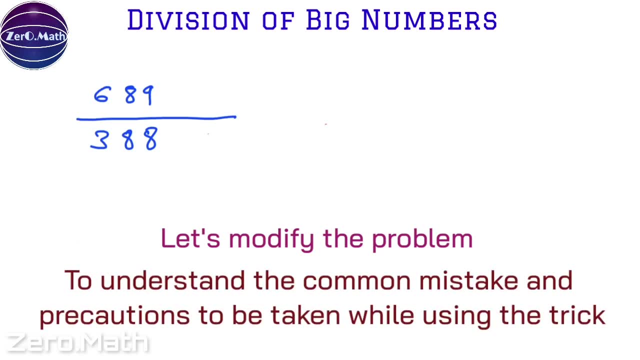 difference is hardly 0.006, which is negligible difference. Now let us modify this problem a bit so that I will tell you what are the precaution that must be taken while dealing with such kind of problem. So what I am going to do. 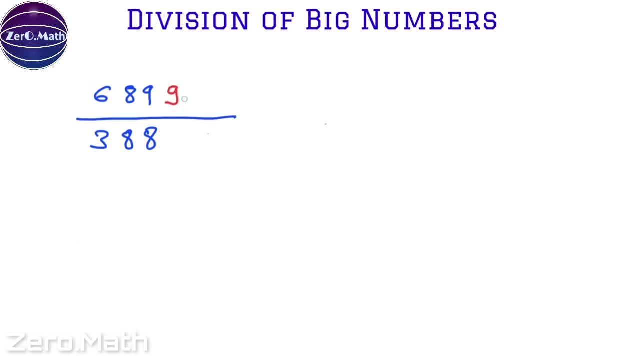 is, I am going to add 1 additional digit over here, So this was 3 digit number by the 3 digit number. Now this will be 4 digit in the numerator and 3 digits in the denominator. Let us solve this problem. as a first step, let us simplify the denominator. So if we 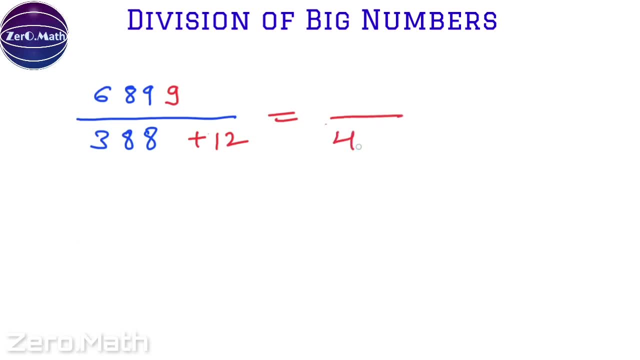 add 12 to the denominator, we will get 400.. So let us write it down. Now question is what we should add to the numerator. To find it out, let us find out the approximate unit value of 6899 by 388.. 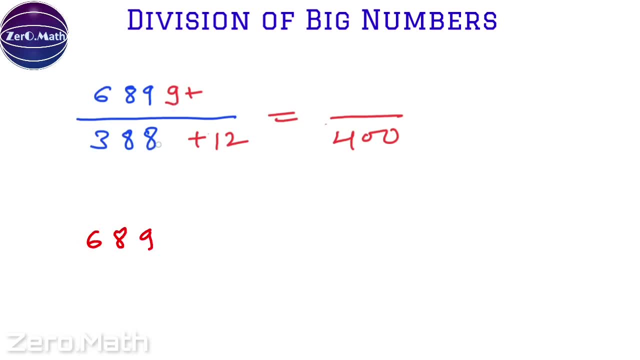 6899, right, Yes, 6899 can be approximated as 7388 as 400. if we divide, we will get a approximate unit value as 20.. So 20 times 12 is 240. let us add it to 6899, we will get 7139.. If we divide it by 400, 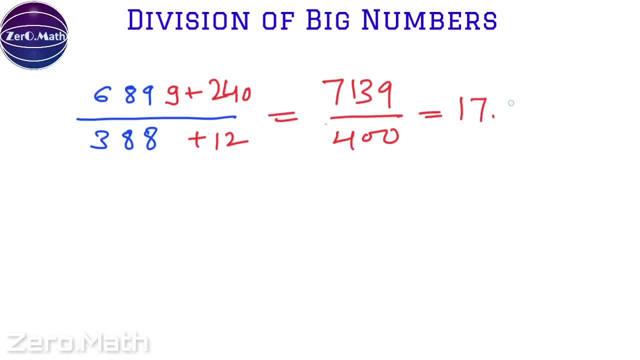 we are going to get 17.8475, which is the approximate answer. Now let us find out what is the calculator answer. So the calculator answer is 17.7809. if you see, the difference between both the answers is 0.0666, which is 10 times the difference when we are dividing 689 by. 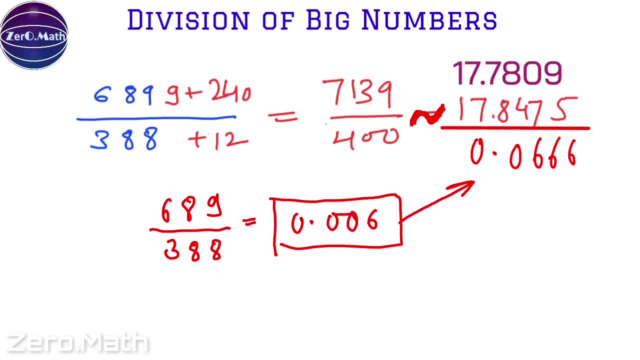 388, which means addition of one digit in the numerator, and your precision is changing almost 10 times. Similarly, if I try to divide 689 by 388, which means addition of one digit in the numerator, and your precision is changing almost 10 times. Lets see how much, what answer we get and what is the difference. SO, 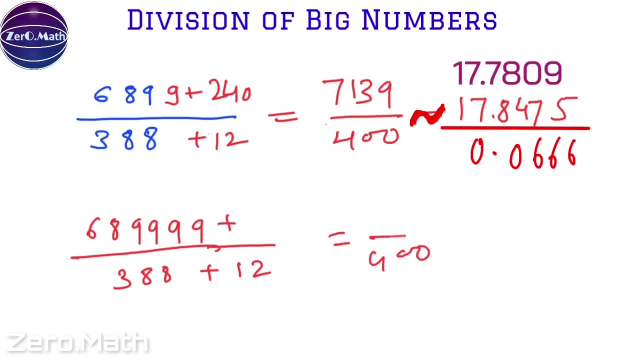 add 12 here, and so this will be 400 in the numerator we have to add 24000, because it will be 12 times this 2000, which is approximate unit value. Now, if we add this, we are going to get 71399. 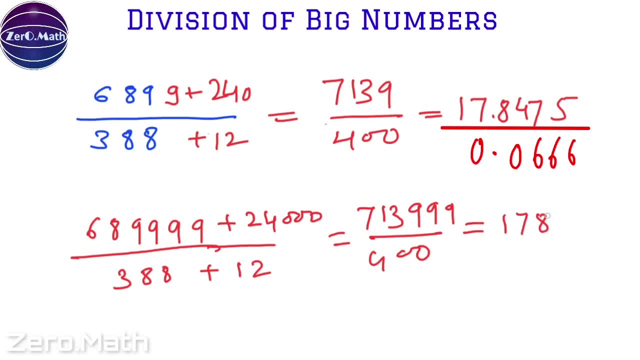 So this is 12 and it is 400.. Now if we subtract from the equation and we multiply, we get, And if we divide it by 400, the answer would be 1784.99.. Now the calculator answer is 1778.34. 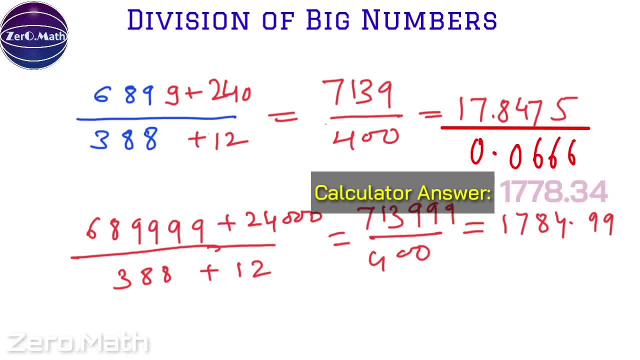 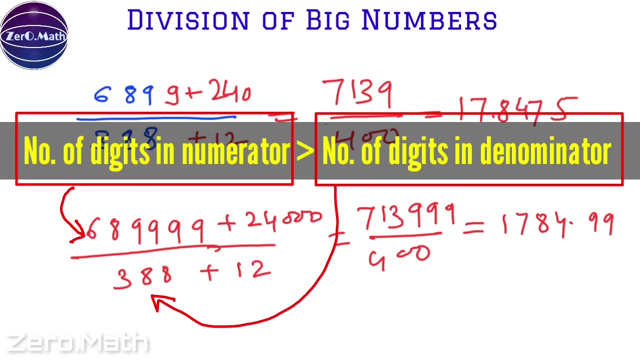 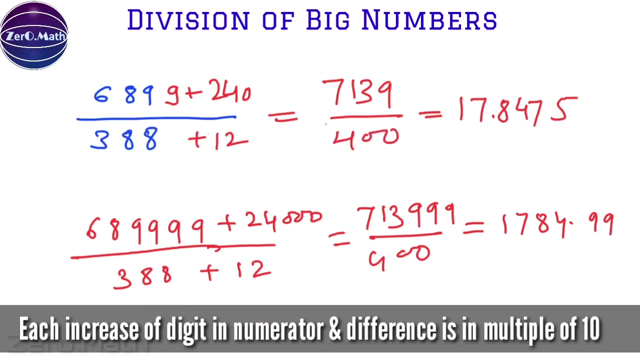 And if you find out the difference between both the answers, it would be 6.06.. What we understand from this is: if the number of digits in numerator are more than number of digits in denominator, then you have to be very, very careful, because each increase in number of digits in numerator is causing your answer, or your approximation, 10 times. 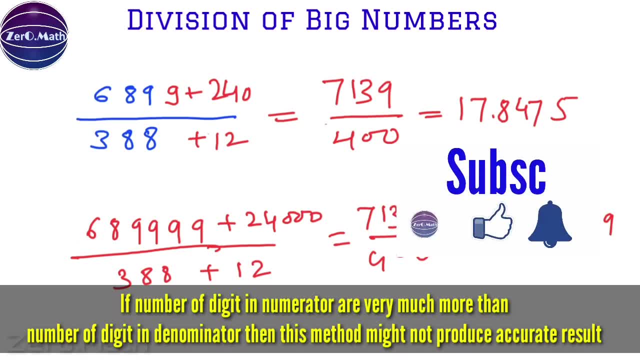 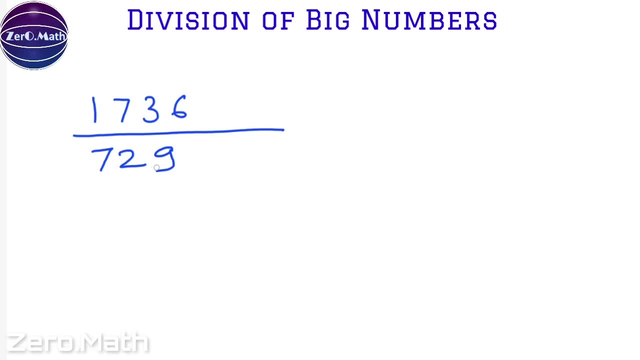 Which means if number of digits in numerator are very, very high as compared to number of digits in denominator, then this method might not give you an accurate result. So keep this thing in mind. Let's try to solve this problem. 1734.. 6 by 729, which is posted by user Crazy Mood Saver. 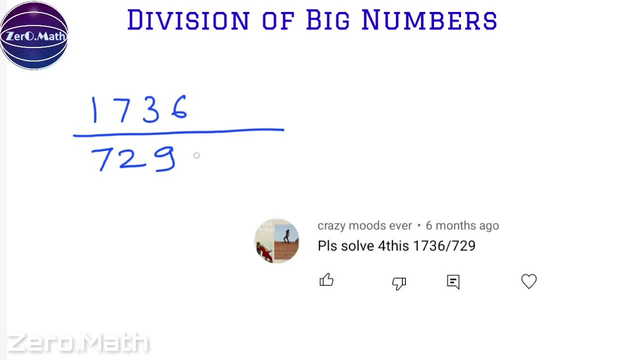 Interesting name. Let's first simplify the denominator. If I subtract 29 from 729,, I am going to get 700.. And division with 700 is easy, isn't it? Now, what should I subtract from the numerator is the question. 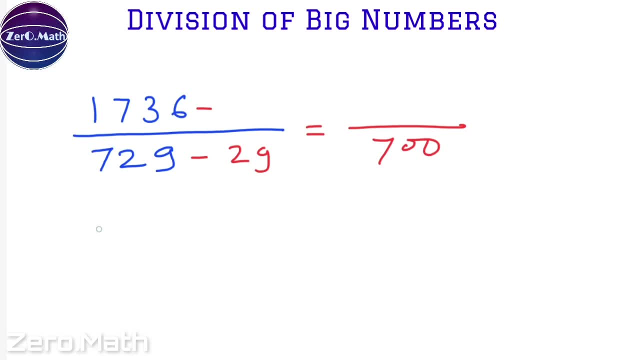 So if I find out the approximate value of 1736, it would be 1700. And approximate value of 729 would be 700. So 1700. So by 700 would be somewhere between 2 and 3.. Because 7 times 2 is 14 and 7 times 3 is 21.. 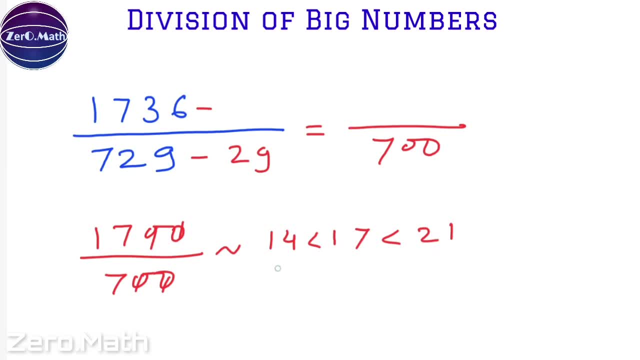 So 17 falls in between 14 and 21.. So if I take approximate value as 2 or 3, that won't be accurate. Rather than that, 2.5 would be a more accurate approximate unit value, And this is something you should understand. 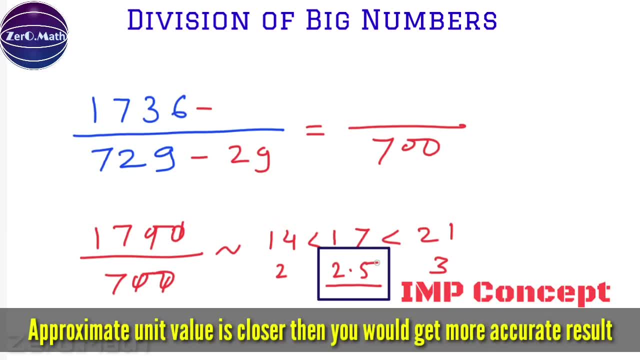 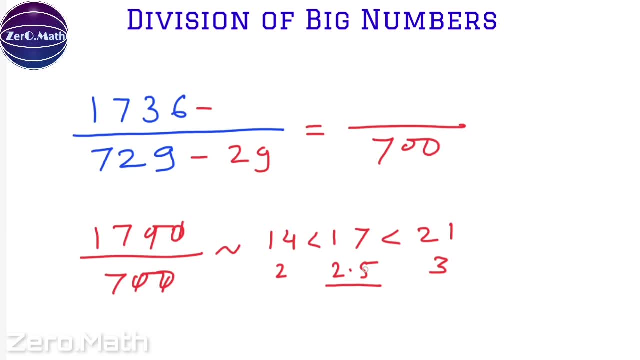 Closer the approximate unit value, closer the answer you are going to get. This is a very important thing you should remember, And this is a common mistake which everyone performs, Like you know how to choose the approximate unit value. So 2.5 times 29 would be 29. times 2 is 58.. 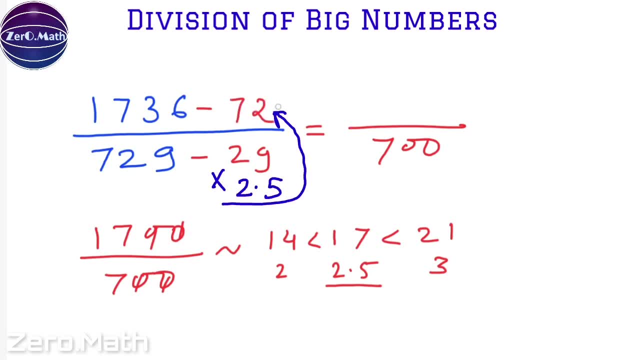 And 29 half would be 14.. So if we do that, 58 plus 14 is 72. And 1736.. 6 minus 72 would be 1664.. Now let's divide 1664 by 700.. 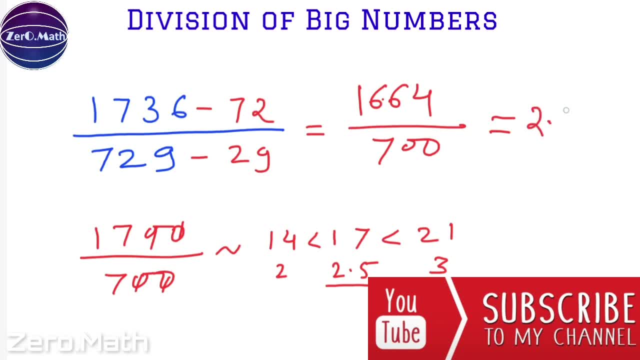 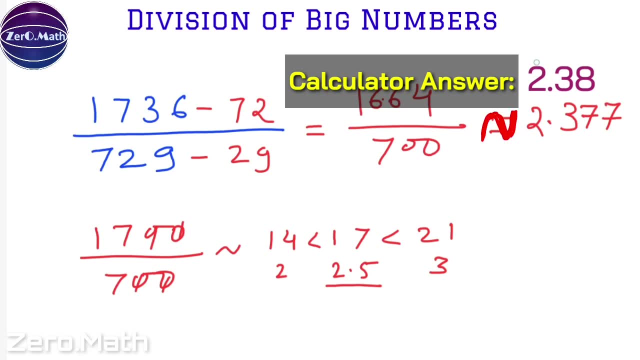 We are going to get 2.377.. And the calculator answer is 2.38.. You can see, there is hardly any difference. The difference is 0.01.. I hope, Mr Crazy Mood Saver, this clarifies your doubt. 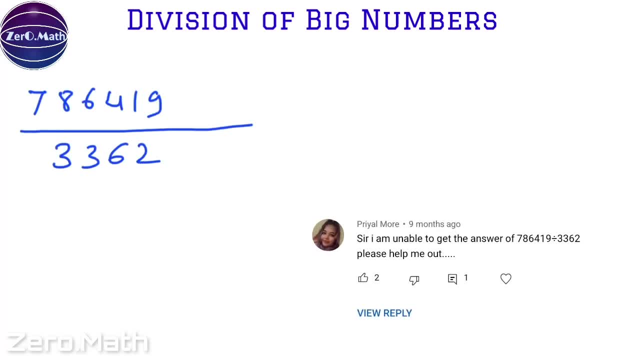 Let's solve this sum posted by user Priyal More. Let's divide this big number- 7, 8, 6, 4, 1, 9- by 3, 3, 6, 2.. First step is to simplify the denominator. 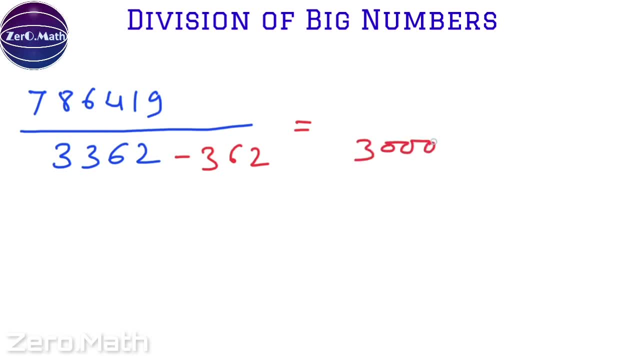 We will subtract 362 from the denominator So that we will get 3000. Which is a simplified form. Division by 3000 is always easy. Now the question is what we should subtract from the numerator To find it out what we will do. 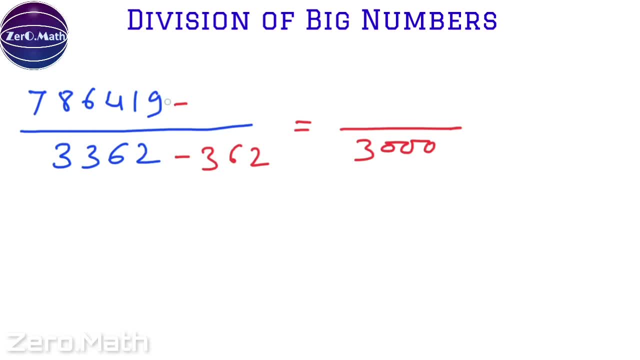 We will find out the approximate unit value. Since this number is quite big, what we will do, We will remove the two digits from right hand side from the numerator as well as denominator. So we will get 7, 8,, 6,, 4 by 33.. 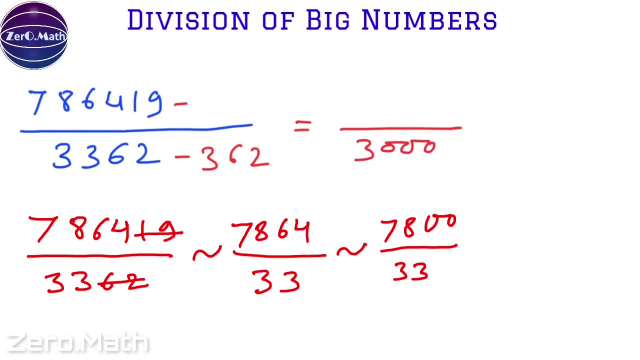 7, 8, 6, 4 can be approximated as 7, 8, 0, 0 by 33.. Now, 33 times 2 is 66 and 33 times 3 is 99.. And 78 is somewhere between 66 and 99.. 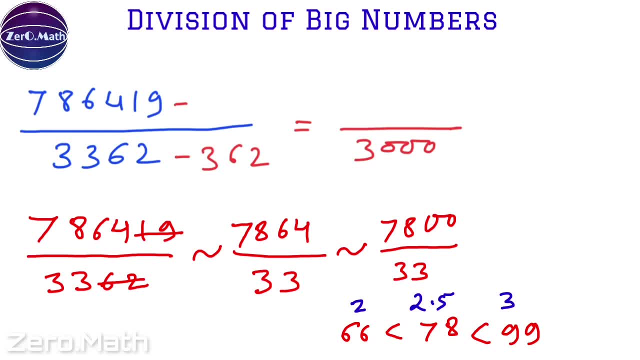 Now the question is: what is the approximate unit value we are going to consider? Is it 2, 3 or somewhere in between 2 and 3, that is, 2.. Since 78 is more closer to 66, we will consider approximate unit value as 2 or 2.5. 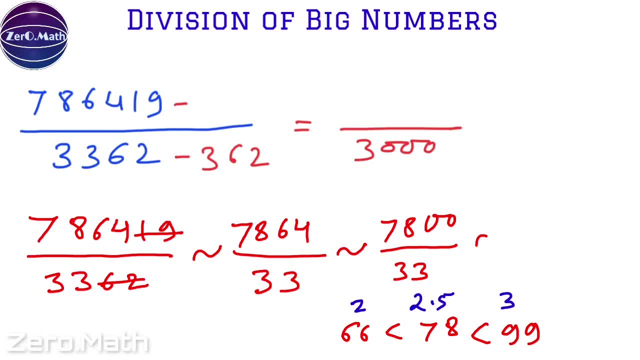 Since we are dividing 7, 8, 0, 0 by 33,, the approximate unit value would be either 200 or 250.. Let's take approximate unit value as 200.. So 200 times 362 is 7, 2, 4, 0, 0. 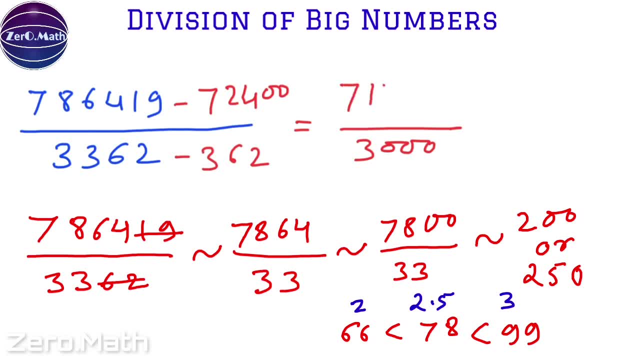 If we subtract it from 7,, 8,, 6,, 4, 1, 9,, we are going to get 7, 1, 4, 0, 1, 9.. Let's divide it by 3000.. 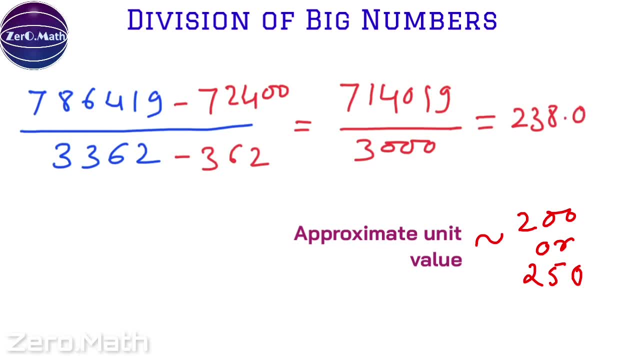 We will get answer as 238.006.. The calculator answer of this sum is 233.914.. If you can see, there is a quite a difference between both of these numbers. Now let's try to use the approximate unit value as 250 and try to figure out what is the answer. 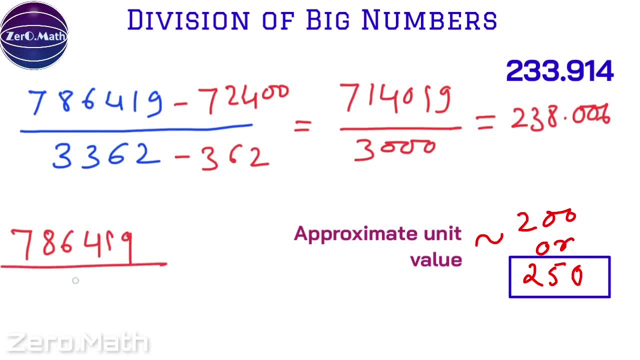 So 7, 8, 6, 4, 1, 9 over 3362.. So let's subtract 362 from The denominator and 362 times 250 from the numerator, So that would be 90500, and if we subtract this we will get 695919 over 3000. 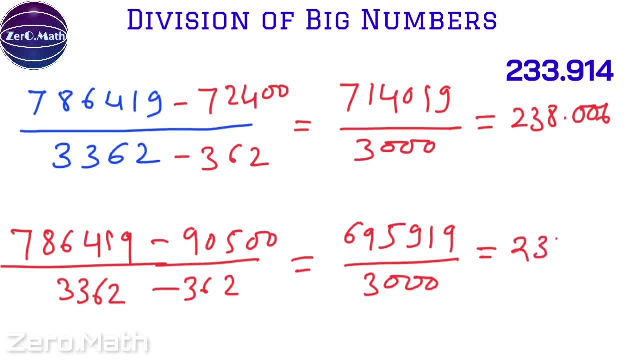 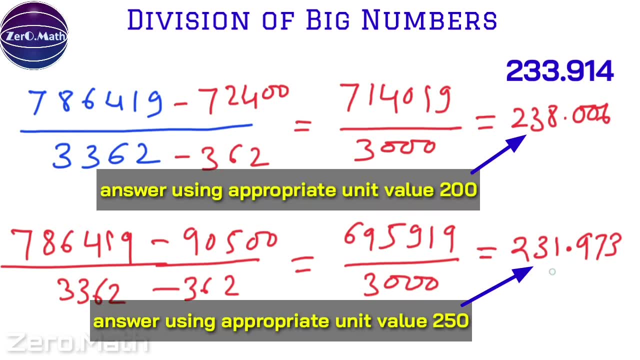 So if we divide this number by 3000, we are going to get 231.973.. Now you can see the difference between the calculator answer. It is very less. It is just the difference of 2.. This is the trick you are going to keep in your mind when you are dividing big numbers.